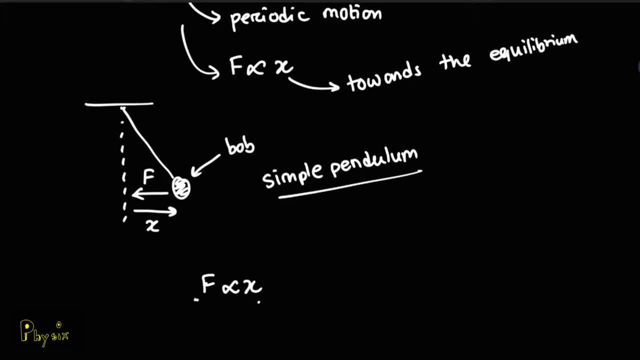 that F is in the opposite direction of its displacement x. So since F and x are in the opposite directions, we can say that F is equal to minus kx, where the minus sign denotes that they are in opposite directions and k is the proportionality constant. 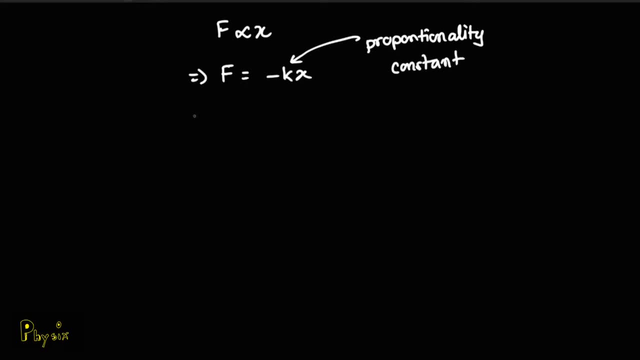 All right. so if the mass of the bob in this pendulum over here, if the mass is m, so we could say that F over here is basically ma right, And this minus kx can be written down as x minus kx. okay. 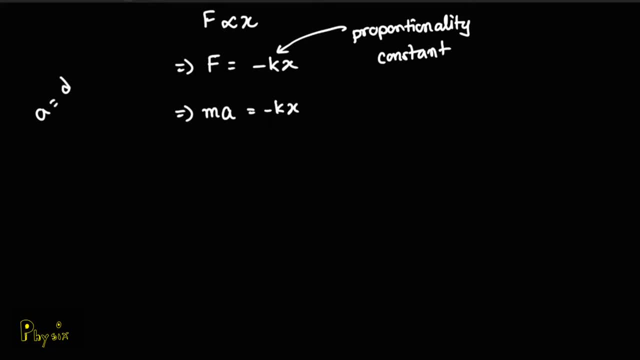 So acceleration right. Acceleration can be written down as the second derivative of the position, function right. So we write it down in this form And we can of course divide both sides by m right. So in physics we say that this thing over here k over m. 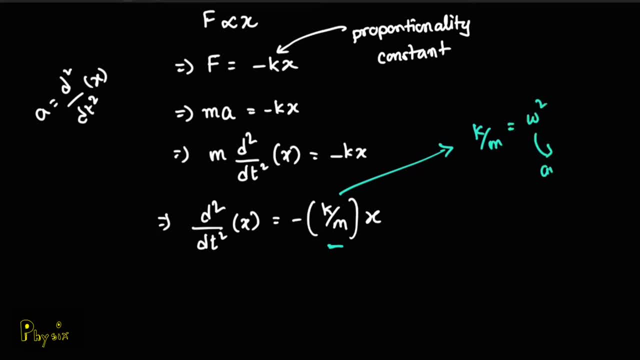 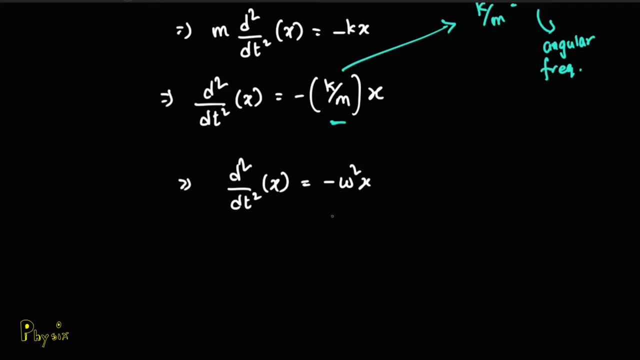 is defined as the square of the angular frequency. So we can write this down as: and if we take this thing into the left side, then we are left with this, And this is the general equation of any system revolving in simple, harmonic motion. 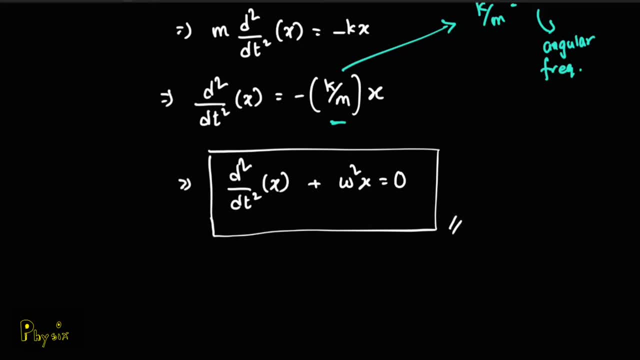 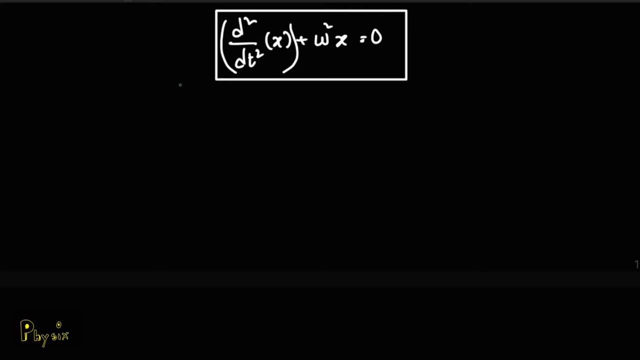 But we actually want to simplify this entire thing. So what do we do? As you can see over here, this entire function over here can be written down as acceleration right. This entire thing is the second derivative of the position function and acceleration is basically the second derivative of the position function. 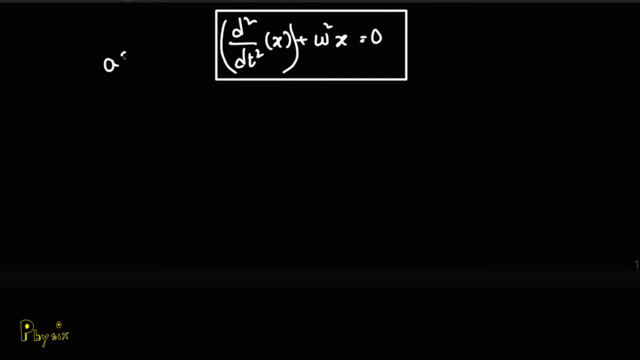 And then again, acceleration can be written down as the first derivative of the velocity function, right? So we can write this entire thing down over here as dv dt plus omega. squared x is equal to zero. And then again, following the chain rule of calculus, dv dt can be written down as dv dx times dx dt, right. 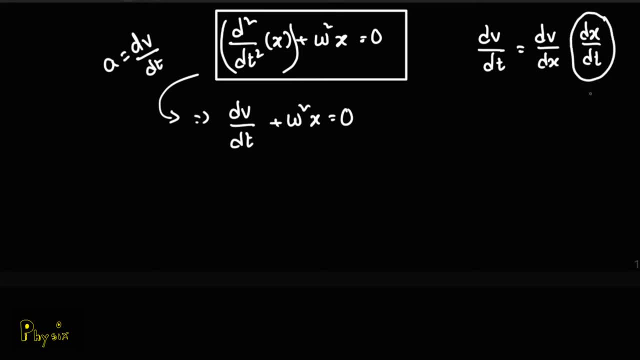 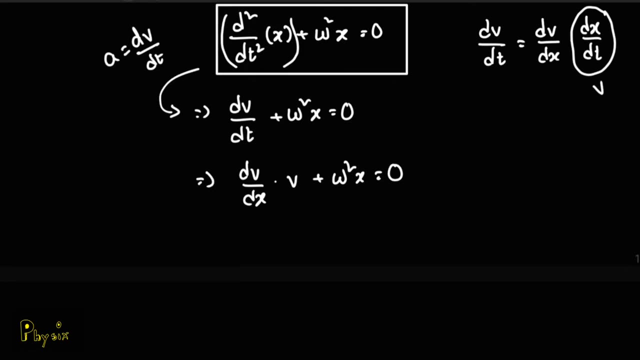 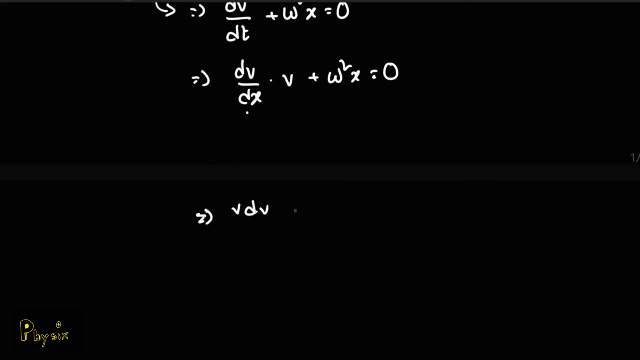 And then again notice that this dx over dt, dx, dt can be set to be v right, Which is velocity. So we write this down as dv, dx. v plus omega squared x is equal to zero, right, And we multiply both sides with this x over here and we are left with dv, v plus omega squared x. dx is basically zero. 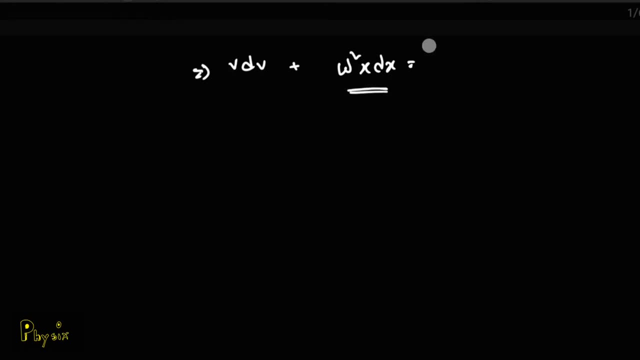 And if we take this thing over here to the right side, we are left with this. And we want to simplify this, We want to integrate both sides And by integrating we are left with- and c is the integrating constant over here. 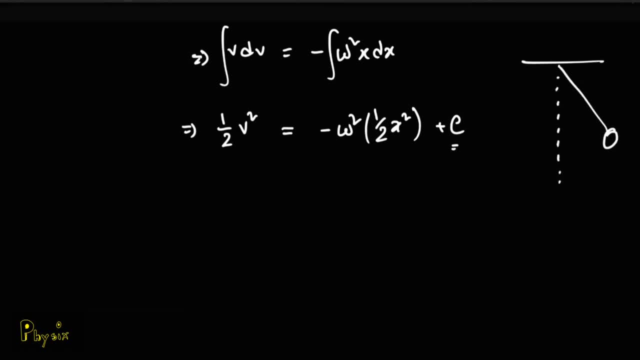 Notice that when we dealt with the pendulum over here, at the maximum displacement, which is x is equal to amplitude, the velocity of the bob is basically zero And putting v is equal to zero at x is equal to a in this equation over here. 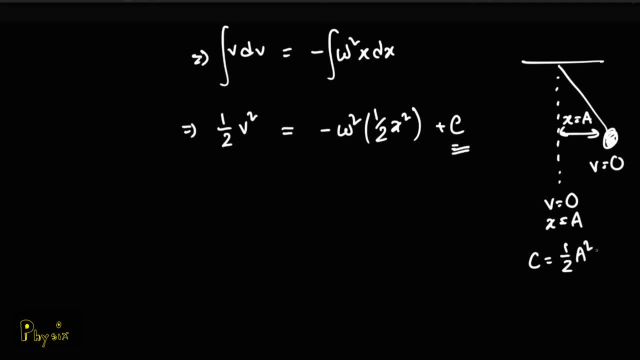 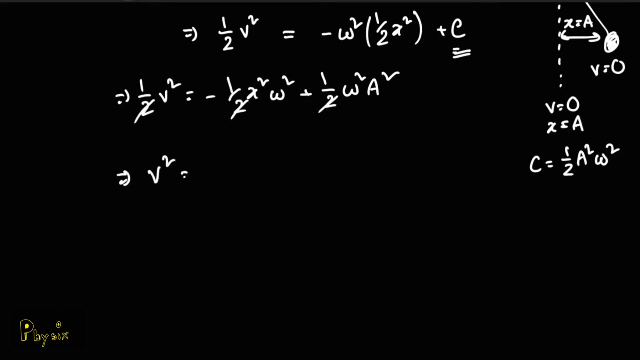 c happens to be half a squared, And then we are left with half v squared is equal to minus half x squared. omega squared plus half omega squared a squared, And we can cancel the twos and the denominator off And we are left with v squared is equal to omega squared times a squared, minus x squared. 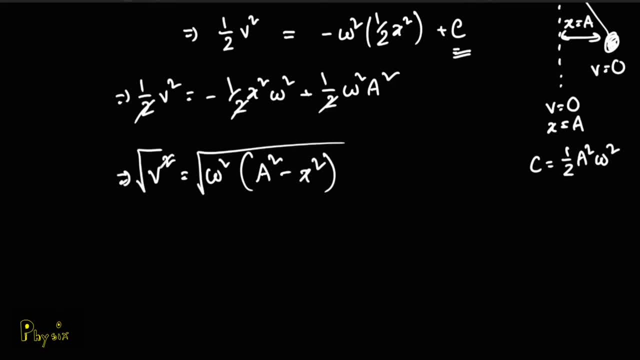 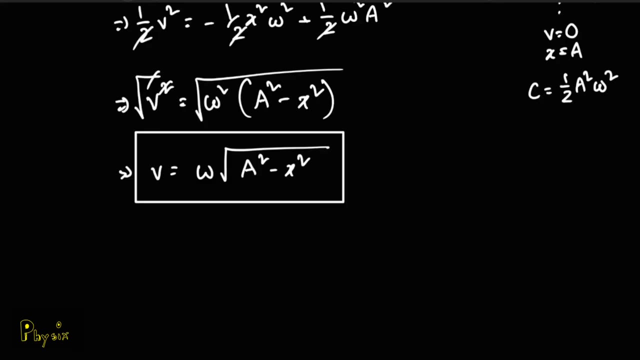 And by taking the square root of both sides, we are left with v. And by taking the square root of both sides, we are left with v squared times a squared minus x squared. But this is the velocity, right? We want to calculate the equation that says its position, right? 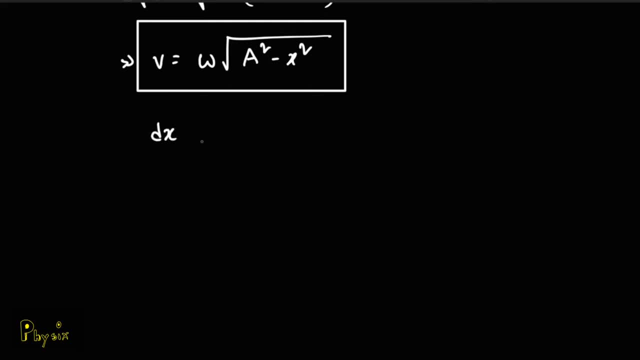 So then again we can write v as dx over dt, But we take the dt in the right side And thus we are left with this equation, right, And then we get to integrate both sides. But integration would be easier If we took this term over here in the left side, because this term over here contains x.